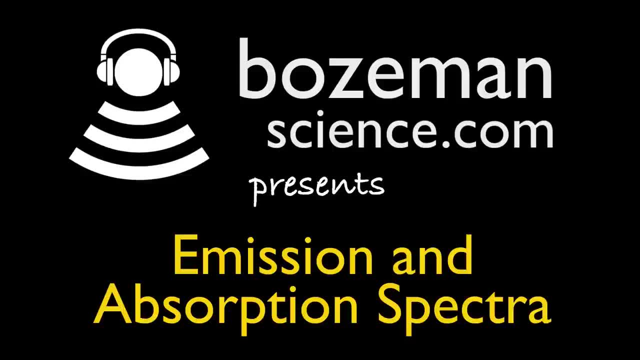 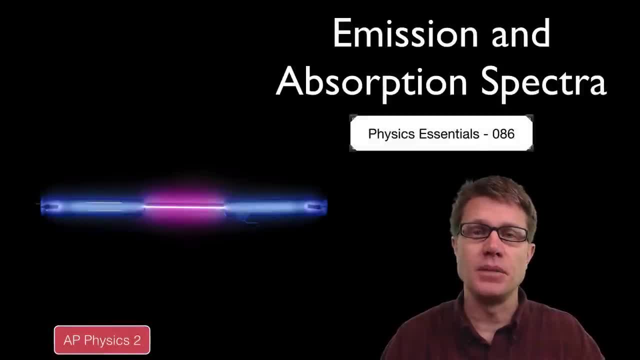 Hi, It is Mr Andersen and this is AP Physics essentials video 86. It is on emission and absorption spectra. If we were to take a gas like hydrogen and put it in a discharge chamber and shoot electrons at it, it is going to give off light that looks like this. If we 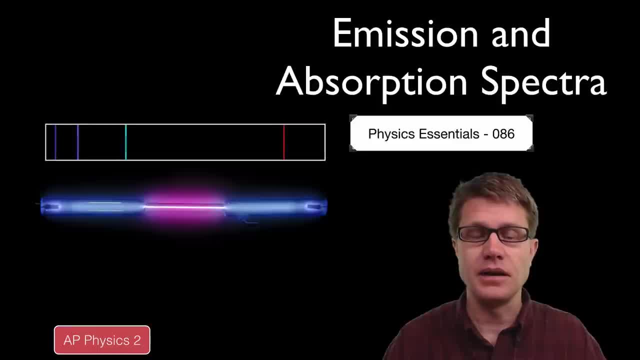 were to analyze that light, if we were to split it in a prism, it would look like this. So, instead of being a rainbow of light, we are going to get these discrete units of light, or these discrete photons that are carrying discrete amounts of energy. And this was puzzling. 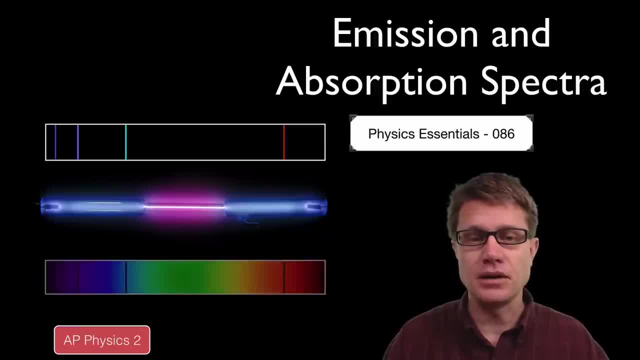 to scientists for a long time. We could also shine light through that discharge chamber, and parts of it would be absorbed, And so this would be the absorption spectra. So most of the light would make through, but some of it is not going to make it through, And this 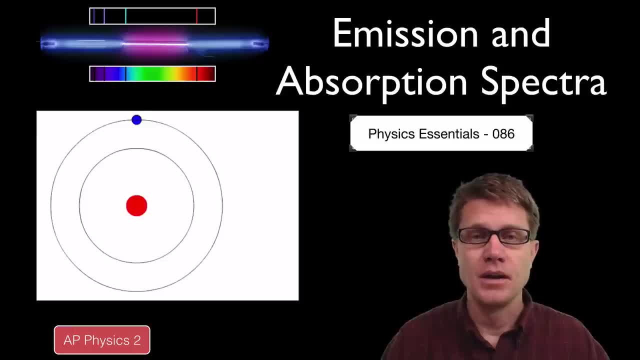 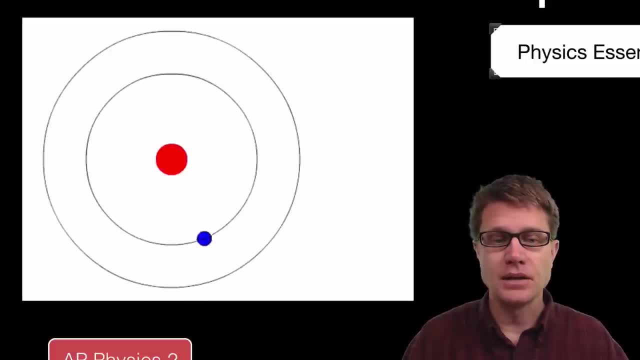 puzzled scientists for a long time, until Niels Bohr finally figured it out. And what is happening if we look at a hydrogen just in the first two energy levels, is that as the electron goes around the atom, as it jumps to a lower energy level, the energy level of the atom. 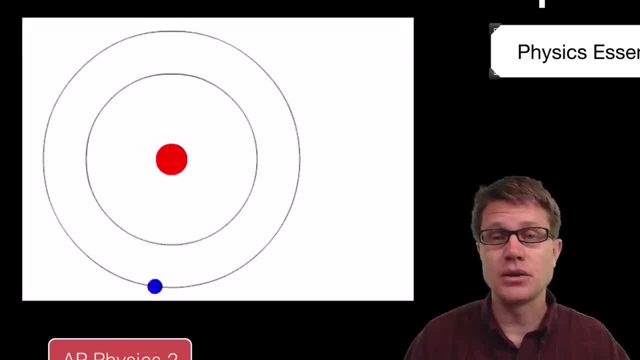 is going to give off a photon of light, And for it to move up to that other energy or that higher energy level, it is going to have to absorb a photon, And so there are discrete colors of light that are required for it to jump up, And as it jumps down it is going. 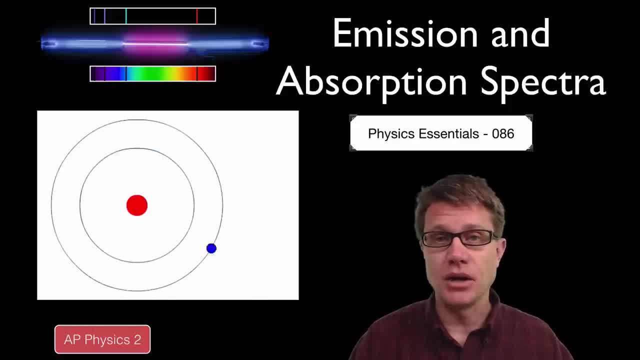 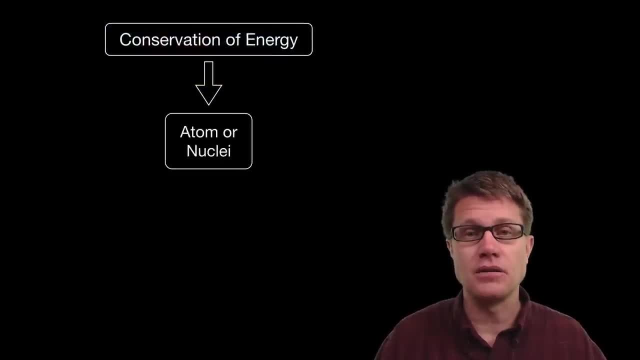 to release these discrete colors of light as well. If you hit it with other colors, it is not going to do anything. It does not have the right amount of energy, And so this is conservation of energy: Conservation of energy in an atom or in a nuclei when it absorbs. 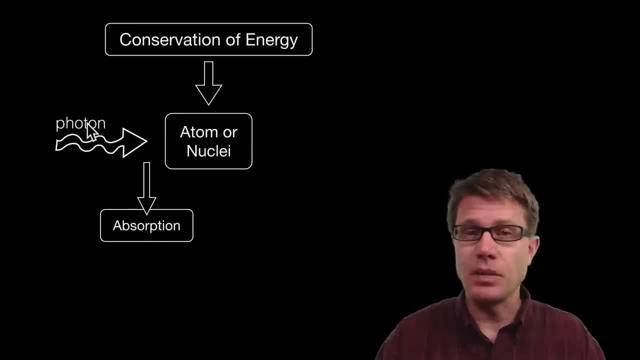 absorbs a photon, So we call that absorption. And so what does that mean? The amount of energy in the photon and the atom or nuclei before absorption is equal to the amount of energy inside the atom or nuclei after absorption, And the same thing applies with emission And 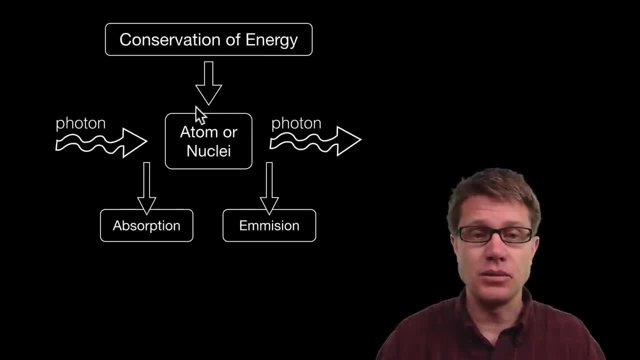 so as we give off that photon, energy is conserved. The amount of energy we had in the atom or the nuclei before is equal to both the photon and atom or nuclei after Now. this is really valuable in science because we could look at what is being given off. So we can look. 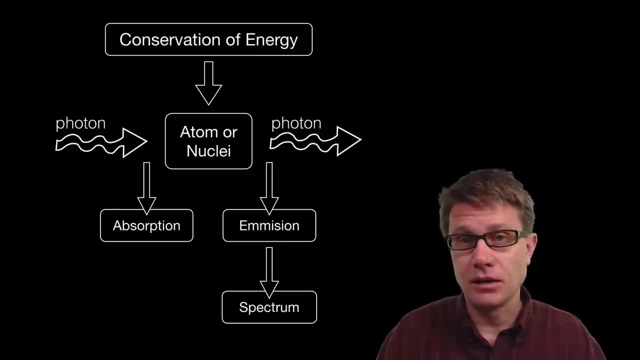 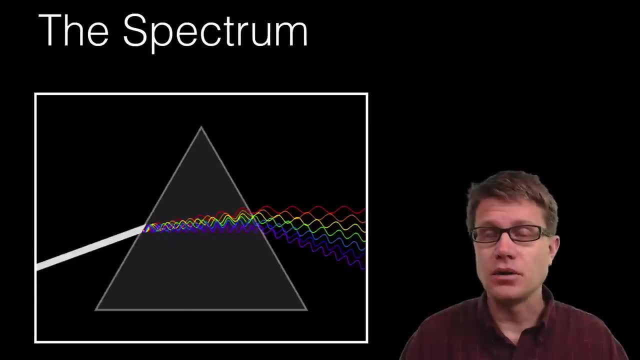 at the spectra of emissions from any kind of element or molecule and it tells us what elements are going to be found inside it, If we know what those energy levels are. And so if you know anything about visible light, it is all the colors of the spectrum. So as 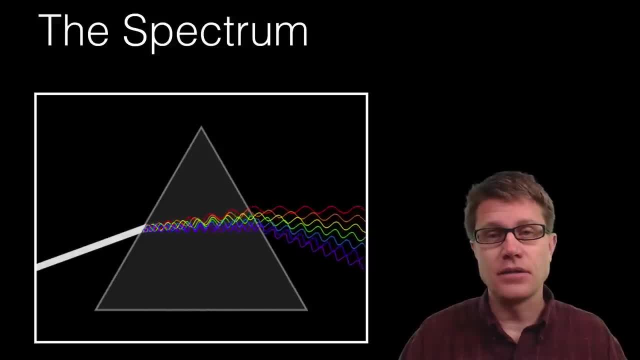 we shine it in a prism. as it moves through the glass, different wavelengths of light are going to travel at different speeds, And so it is going to split it into this spectrum. Now know this: that on the red side, there is a part of the spectrum that we cannot see. 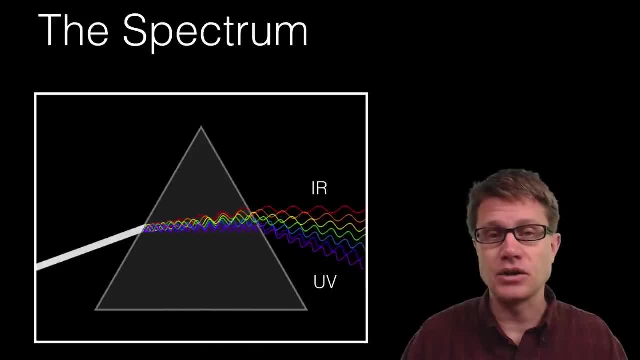 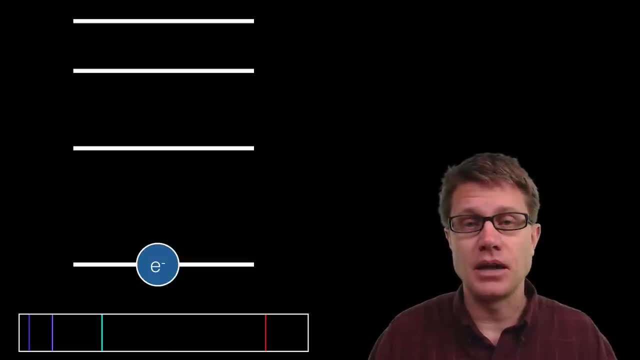 that is infrared light And there is going to be UV light on the other side And we are just seeing that visible spectrum that is going to be right in the middle. And so if we look at those energy level diagrams, for example in a hydrogen atom, if we were to hit it with the right color of photon, so let's shine. 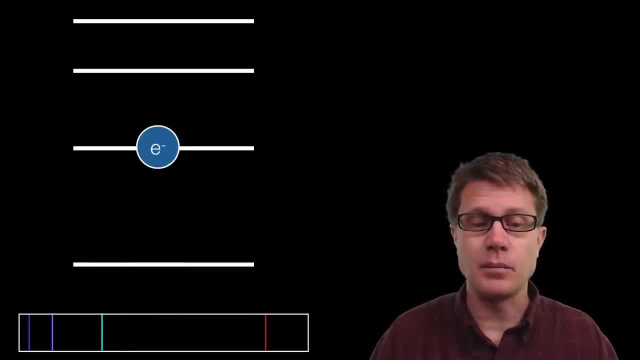 on it the right color of photon, let's say a red photon. watch what happens when it hits that electron: It jumps to a higher energy level. Now, let's say it falls down to a lower energy level. What kind of color is going to be given off from that electron? It is. 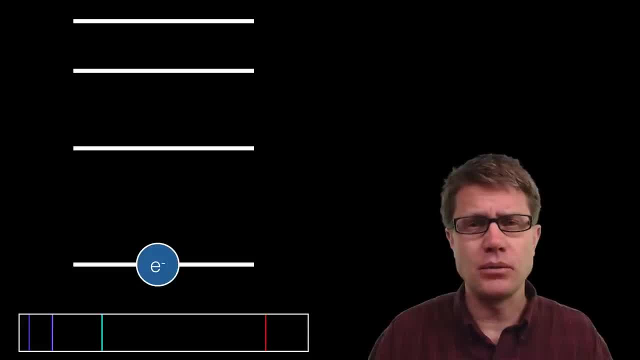 going to be that red photon. But what happens if we hit it with a green photon, for example, and it does not have the right color, does not have the right energy? it is never going to be able to move. Let's say we hit it with a yellow photon. What does it do? Again nothing. And so these atoms. 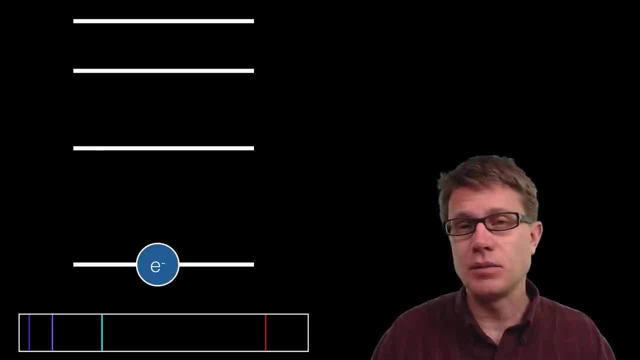 are being bombarded by different colors of photons, but it has to be the right color. Let's say it is the right purple color. What is going to happen? It is going to jump to a higher energy level. What happens as it falls down to that ground state? It is going 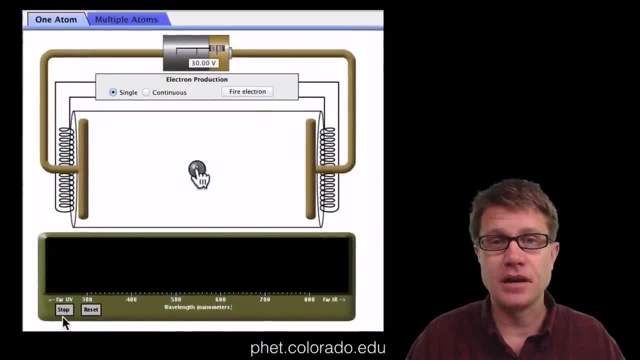 to give off that same exact photon. This is a PHET simulation. What I am going to do is take one hydrogen atom, put it in a discharge chamber. I am going to use a cathode ray to hit it with an electron And watch. 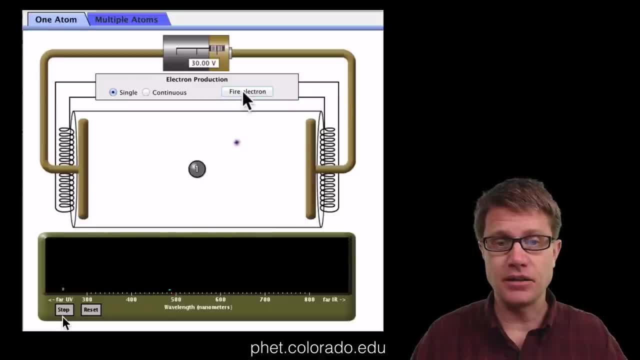 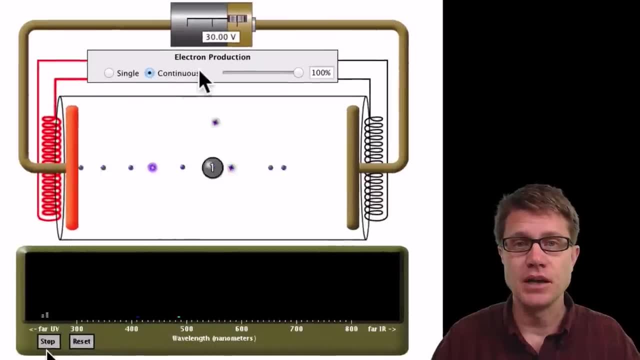 what happens? It gets high energy and as it falls back down, it gives off a certain color of photon. Now, if I were to hit it with not just one electron, but a continuous stream of electrons. before it is able to fall down again, it is giving off different colors of. 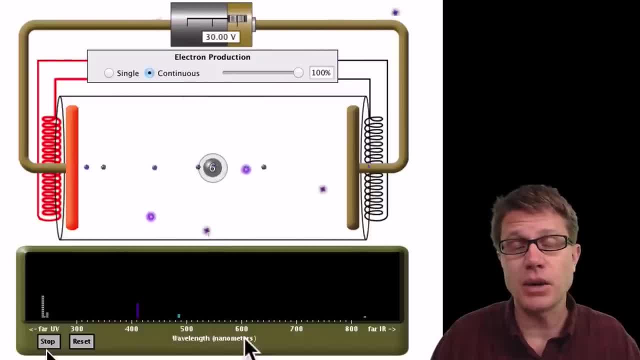 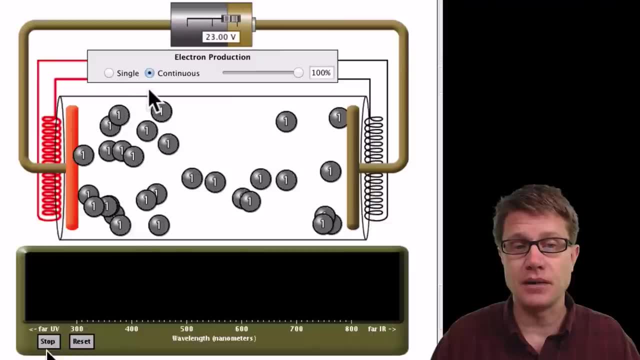 photons. So we are getting all of these different colors of photons And you can see on the spectrum on the bottom of this page it is kind of plotting what color those photons are going to be. So now let's do multiple atoms, Let's do a bunch of atoms. We are going to hit those.